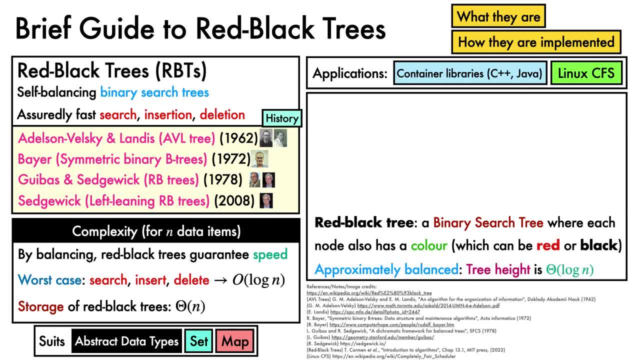 either red or black. It is approximately balanced. The tree height is big. theta of log n. Here is an example Of a red-black tree. you can see that it looks like a standard binary search tree For any node. the left subtree contains keys less than or equal to it. 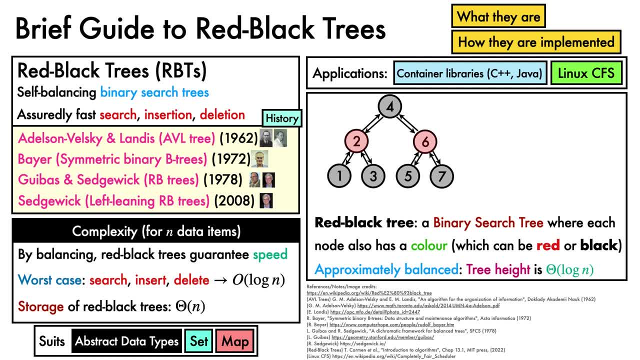 and the right subtree contains keys greater than or equal to it, But this time we have colours. In addition to looking cool, we'll see later that these colours will help us to keep the tree balanced. For cases when a node has either no left child or no right child, it instead points. 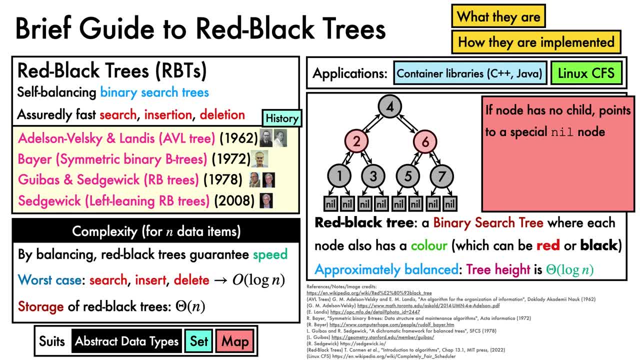 to a special nil node, which can be thought of as a leaf node, whose key value- parent, left child and right child attributes- can be set to arbitrary values. From a colouring perspective, the nil nodes are treated as black. The purpose of these nil nodes is to simplify the logic involved in certain operations. 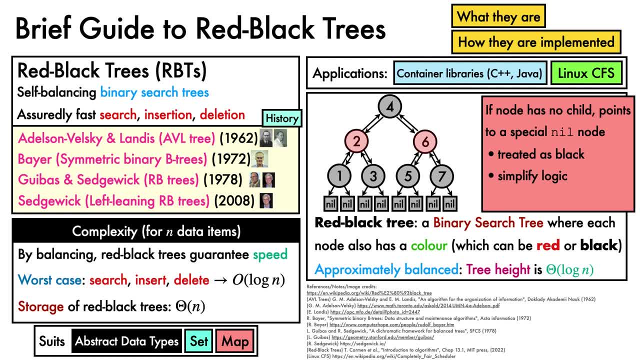 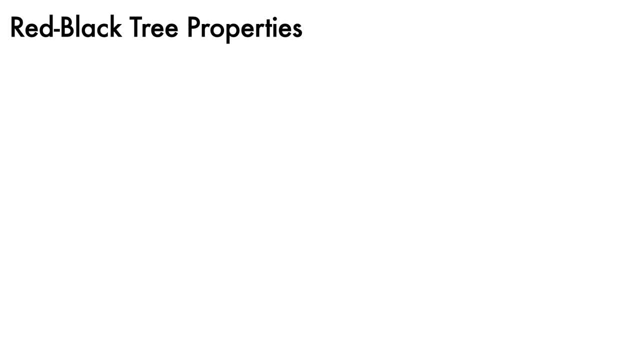 However, since we assume that every node without a child really has a nil node child, we will omit the nil nodes from our diagrams to prevent them from becoming too cluttered. There are several popular ways to define red-black trees. We will follow CLRS, which defines red-black trees as: 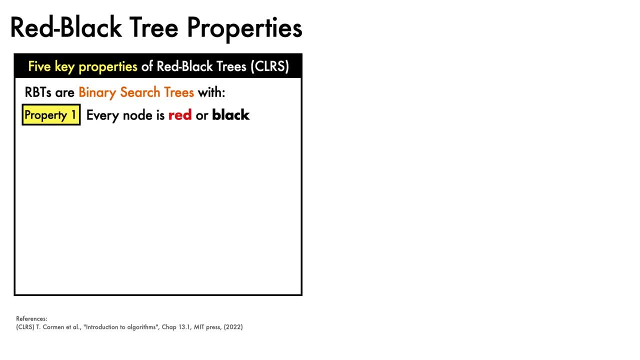 binary search trees with five key properties: Property 1. Every node is red or black Property. 2. The root node is black. Property 3. Every leaf node which we've just seen is a nil node is black Property. 4. If a node is red, both of its children are black. 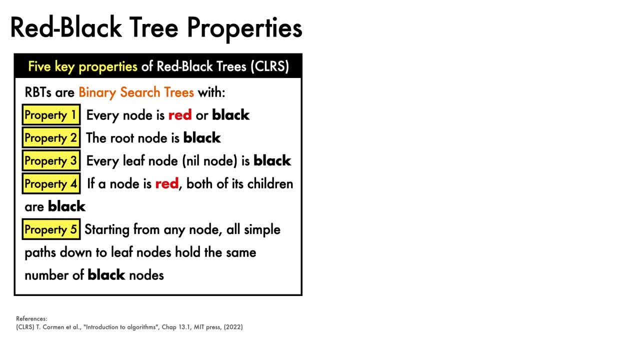 Property 5. Starting from any node in the tree, all simple paths down to leaf nodes hold the same number of black nodes. These properties may seem somewhat arbitrary, but they have useful and important consequences. With these properties we can show that the height of a red-black tree is big. theta of log n. 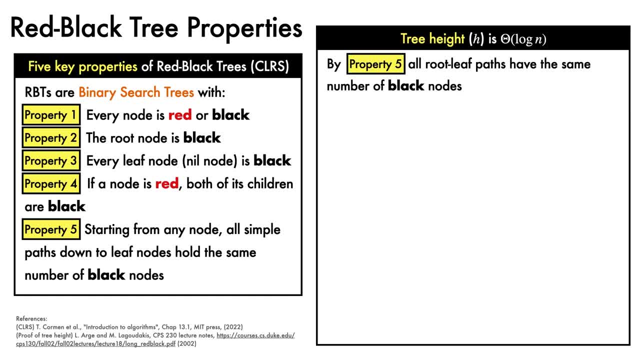 which implies that it's fairly well balanced. By property 5, we know that all paths from the root to a leaf have the same number of black nodes. And by property 4, we know that all red nodes must have black children Together. these imply that the longest path from the root to a leaf 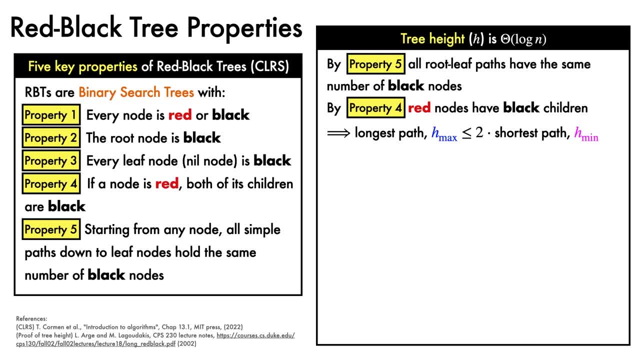 ie the maximum height of the tree is less than or equal to twice the length of the shortest path from the root to a leaf, ie the minimum height of the tree. A useful fact to note here is that a complete binary tree 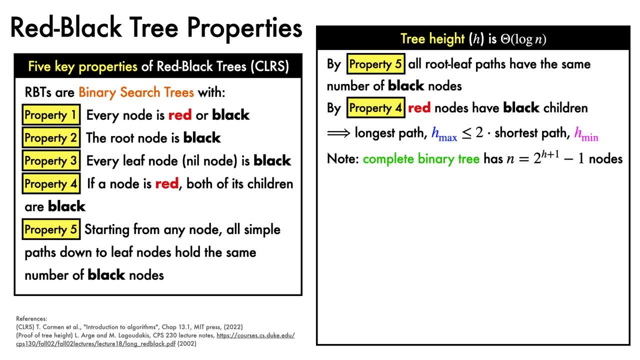 where every internal node has two children, has 2 to the h plus 1 minus 1 nodes, where h is the height of the tree. For example, a complete binary tree of height 0 has at most 1 node, because 2 to the 1 minus 1 is 1.. 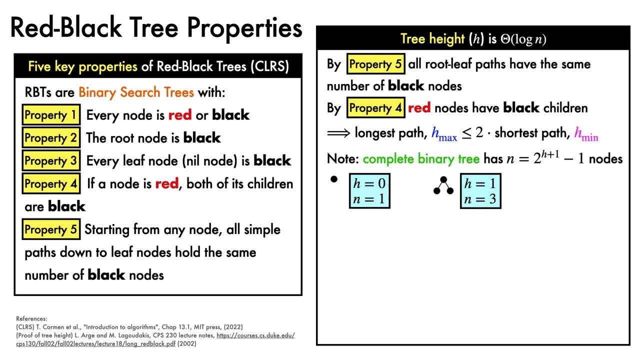 A complete binary tree of height 1 has 3 nodes, because 2 to the 2 minus 1 is 3.. A complete binary tree of height 2 has 7 nodes, because 2 to the 3 minus 1 is 7, and so on. 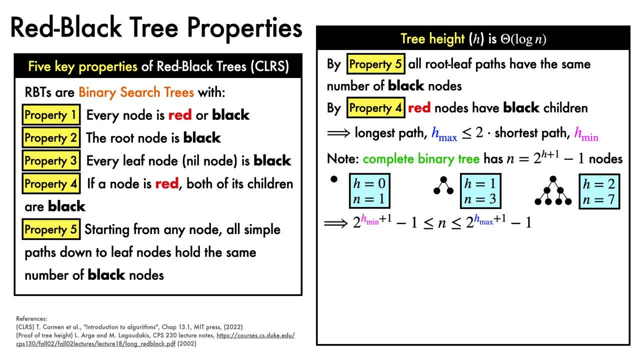 This tells us that the total number of nodes n in the tree must be somewhere between 2 to the h plus 1 minus 1, and 2 to the h plus 1 minus 1.. We can rearrange this equation by adding 1 to each term. 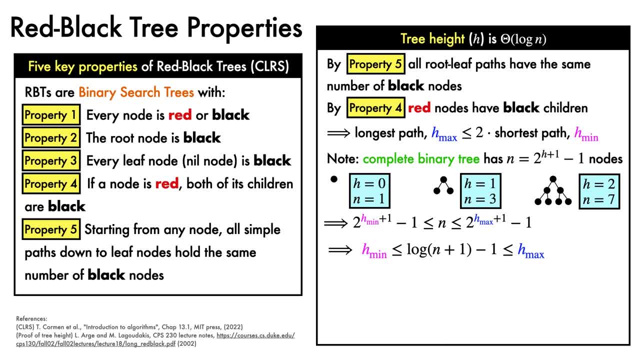 taking logs and subtracting 1 to yield that h is less than or equal to log of n plus 1 minus 1, which is less than or equal to h. From our observation above, we know that h is less than or equal to 2 times h. 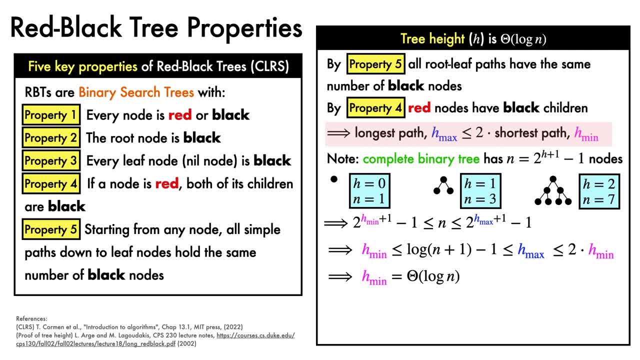 Together, this tells us that h is big theta of log n. Finally, since h lies between h and 2 times h, we also have that h is big theta of log n. This is the key balance tree result. It tells us immediately that operations that rely on tree height and do not modify the tree, 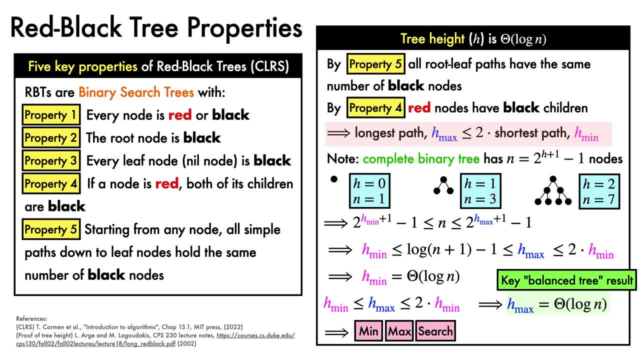 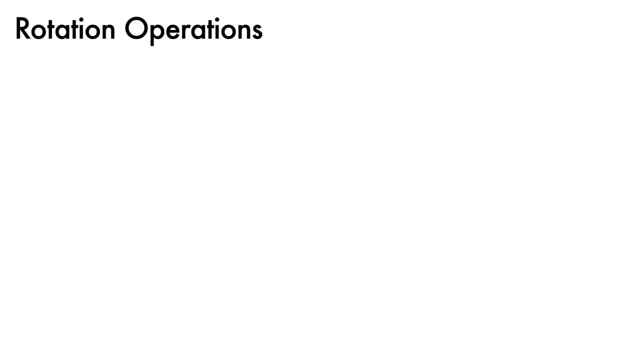 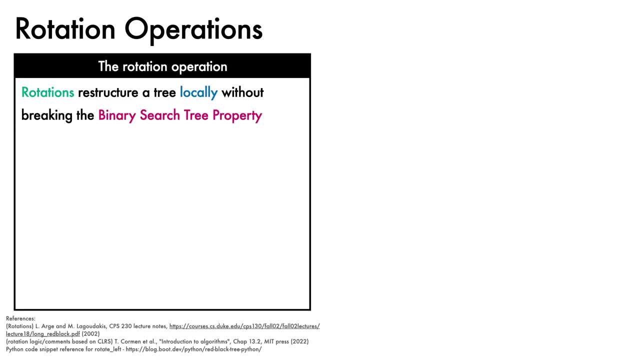 like finding the min and finding the max search, successor and predecessor operations are all big O of log n. We'll now turn our attention to the insertion and deletion of nodes. For that we need to learn about rotations. Rotations are operations that restructure a tree locally. 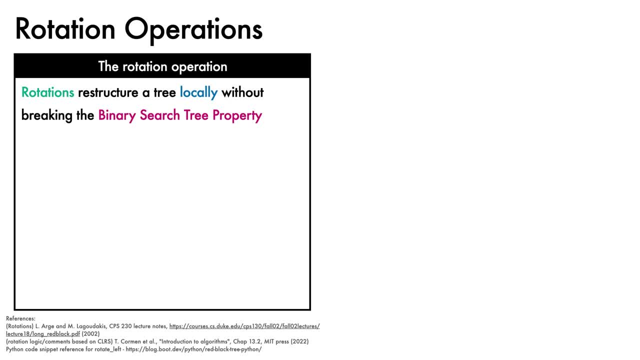 without breaking the binary search tree property. They work by changing links at constant time cost. Note that they do not change red and black colours. We'll do that separately. Now suppose that we have part of a binary search tree that looks like this: 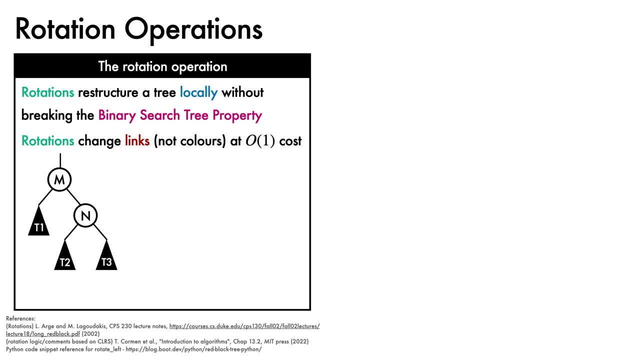 Here we're drawing pebbles. We'll use parent and child links as single lines for simplicity. By assumption, m is less than or equal to n because of the binary search tree property. Below these nodes we are showing subtrees labelled t1,, t2, and t3.. 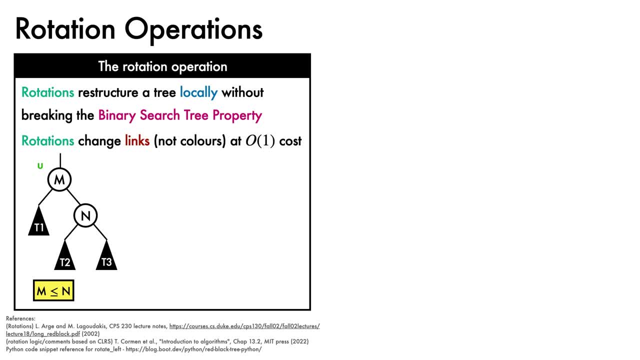 We'll use u to refer to the node with key m, A left. rotate acts on a binary search tree in a particular node, u, by rotating the link between it and its right child, then shifting across subtree t2.. It looks like this: Crucially, we see that the binary search tree property is preserved. 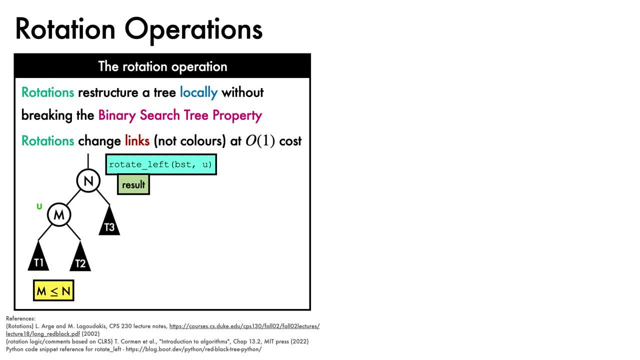 m is still to the left of n, and t1,, t2, and t3 all stay in valid order relative to these nodes. The operation is symmetric in the sense that, given the result of applying left rotate and denoting the node with key n as v, 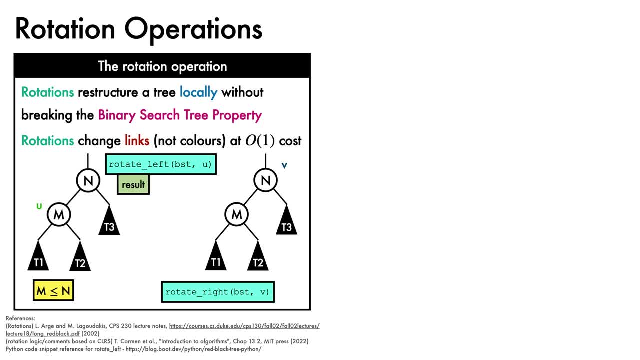 we can apply a right rotate operation on the tree with node v as an argument, which returns us to the original structure. Let's step through a rotate left implementation as a method on a binary search tree. We'll use the binary search tree class in python to understand the operation in more detail. 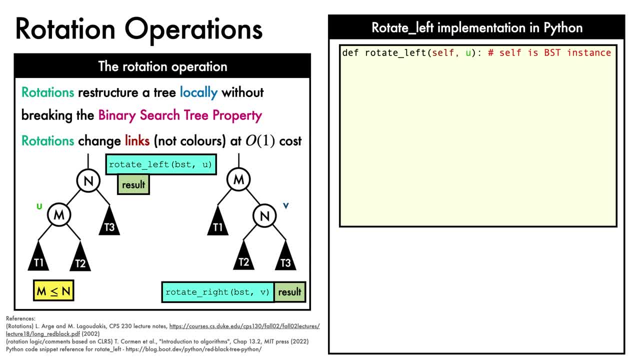 Our function takes in a binary search tree instance and the node u, that will be the target of the rotation. We'll assume that the part of the tree we're focusing on looks like this. The first thing we do is assign the variable v to the right subtree of u. 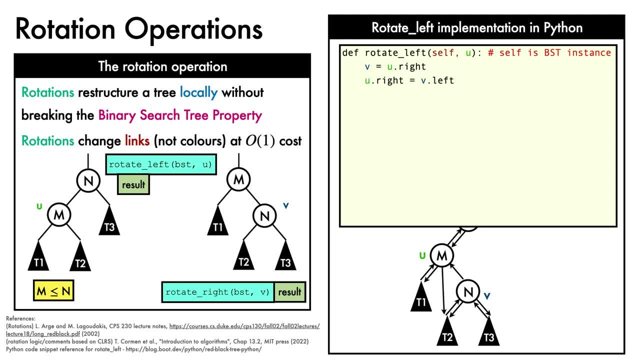 Next, we replace u's right child with v's left child, labelled here as the subtree t2.. When the subtree t2 is not empty, we reattach its parent to u. In our next step, we'll assign the variable v to the right subtree of u. 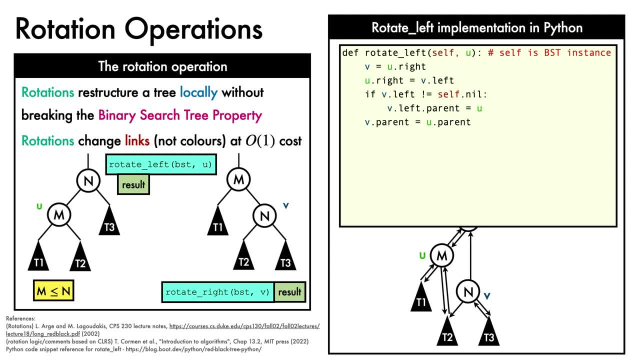 In our next step, we make u's parent v's parent Next. if u was the root, we would make v the root, But it isn't, so we don't. We then check if u is a left child. Since it is, we reassign its parent's left child link to v. 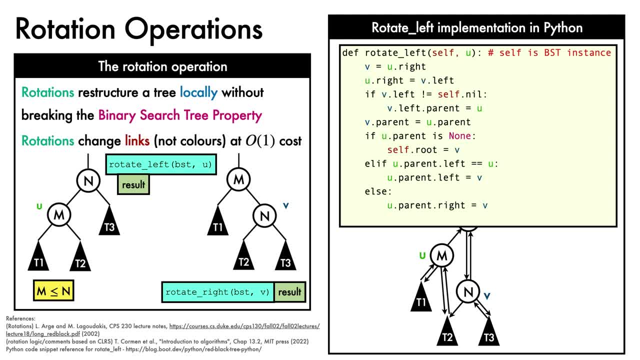 If it was a right child we would do something similar, But it isn't in our example, so nothing is done here. Finally, we reattach the links between u and v, shifting components around to account for the new links. Ok. 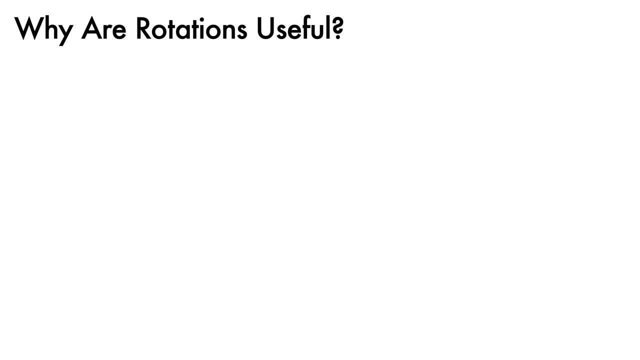 So it's all very well that we have these fancy rotation operations, But why are they useful? The key benefit is that when we have too many nodes on a single path, rotation will distribute nodes to neighbouring paths. This restores balance in the tree. 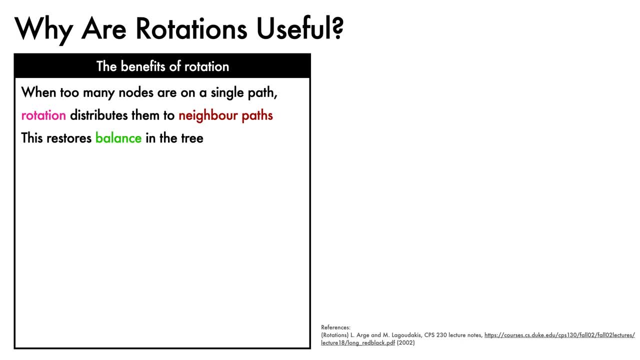 And balance is what we want. Importantly, it does this while preserving our precious binary search tree property. It's easier to understand this rebalancing if we zoom out a little more and consider a chain of three nodes with keys m, n and 1.. 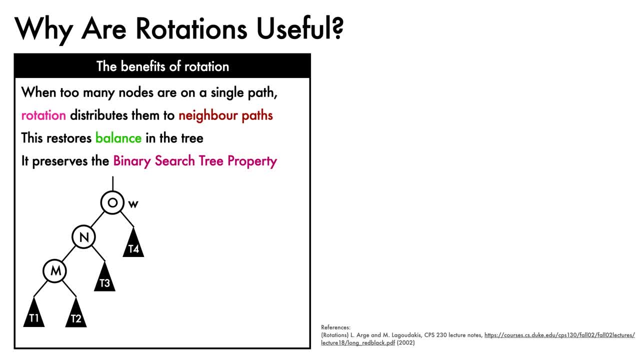 n and o and their subtrees t1,, t2,, t3, and t4.. We've used w to denote the node with key o. This is the kind of chain we want to avoid in a balanced tree. We'll first duplicate the structure for. 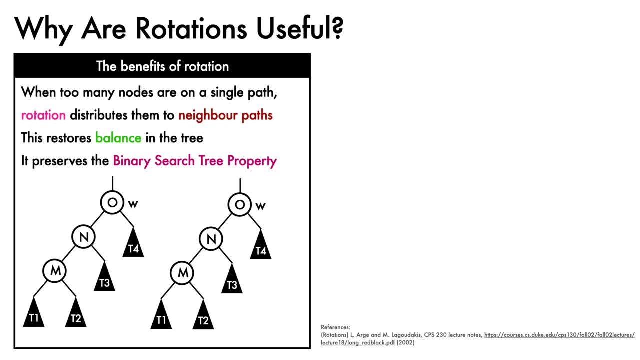 clarity so that we can keep track visually of what is changing. Applying a single right rotation to w produces the kind of balanced structure that we want. This process is sometimes referred to as a single rotation, since it involves a single application of the rotation operation. If we had 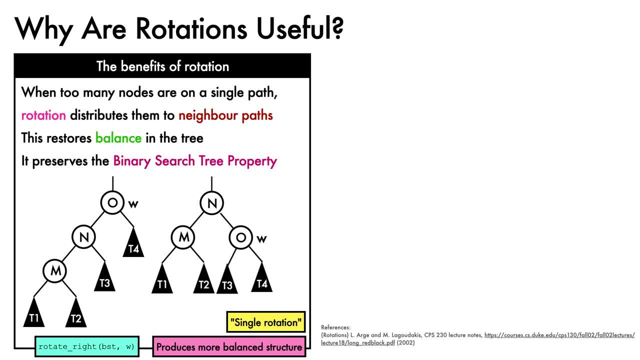 instead started with a right-leaning chain, we could use rotate left rather than rotate right to balance it. For scenarios in which we have a chain with both a left child and a right child, then we need to perform a double rotation. Here is an example of just such a chain We've used. 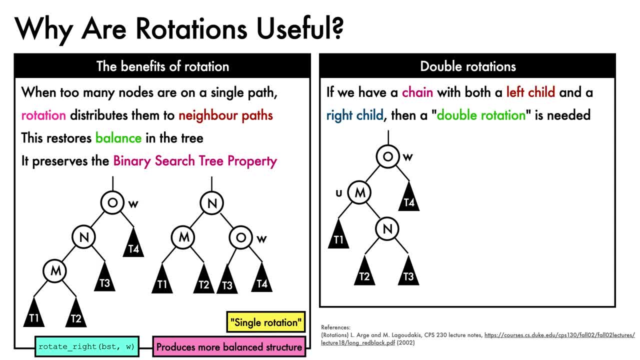 w to denote the node with key o and. u to denote the node with key m. u is the left child of w, which in turn has a right child. We duplicate for clarity To balance this subtree while preserving the binary search tree property. we first call: rotate left on the tree with u. 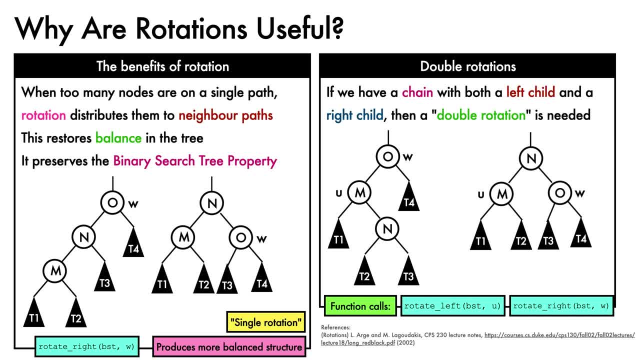 as an argument, Then we call rotate right on the tree with w as an argument, And voila, we have a flatter tree. If we had wanted to flatten a horizontally reflected version of the original chain, we would call rotate left and rotate right, in reversed order. 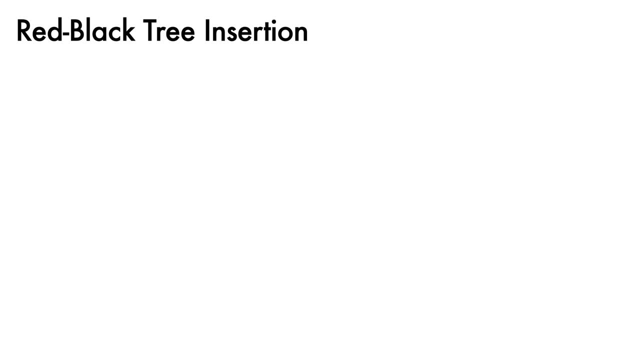 Now that we have the tools in place, we can talk about insertion in red-black trees. Red-black tree insertion starts out identically to the insertion procedure used in binary search trees we saw previously. You can find a link to this in the video description if this is unfamiliar. However, once we've performed our standard binary, 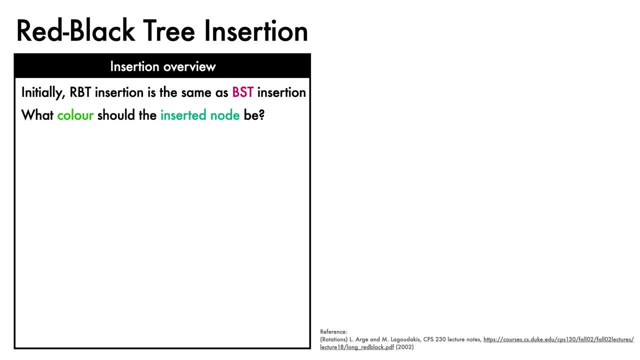 search tree insertion. we must face the tricky question of what colour we should assign to the inserted node. Clearly we have two options: red or black. but we have to be careful. If we colour the inserted node red and we've attached the insertion procedure to the inserted node, we 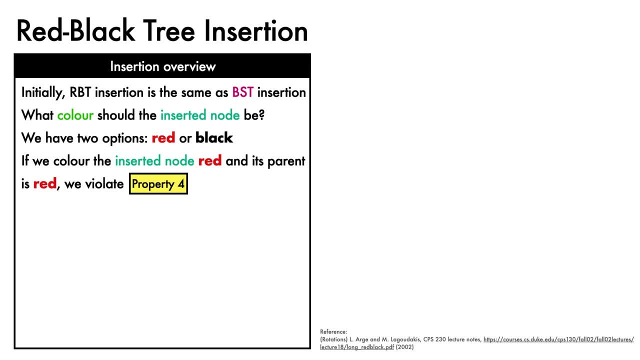 have to attach it to a red parent, Then we violate property 4, which said that red nodes must have black children. If we colour the inserted node black, this node will increase the number of black nodes along paths from the root to the nil nodes below it, so that these paths no longer 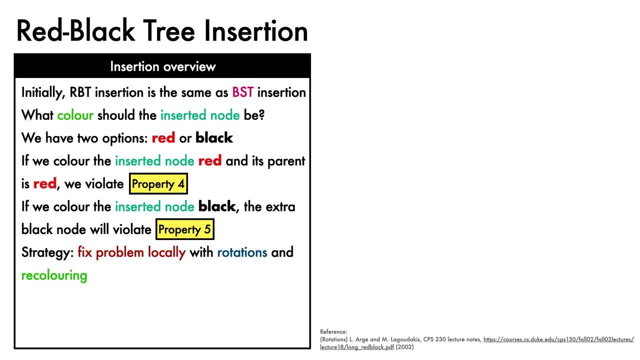 match the others in the tree, violating property 5.. Our strategy to deal with this is to fix the problem locally by using a mix of rotations and node recolouring, and to escalate the property violation issues up the tree if we can't fully resolve them. I like to think of this as a 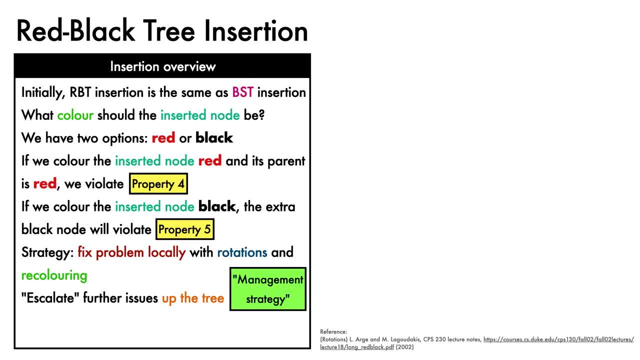 kind of management strategy used in human organisation: If you can't fully fix something, pass it on to the higher ups. Crucially, since the height of a red-black tree is big theta n and each time we escalate we go up two levels, the cost of this escalating and fixing is big O. 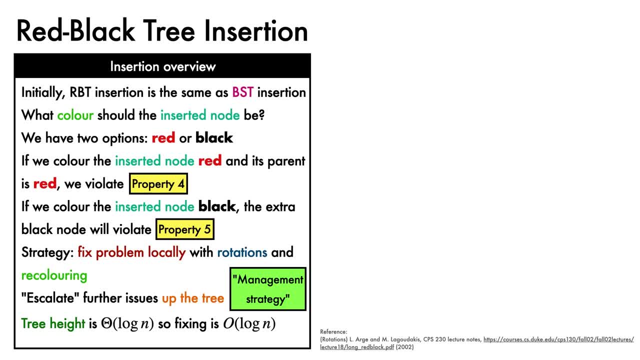 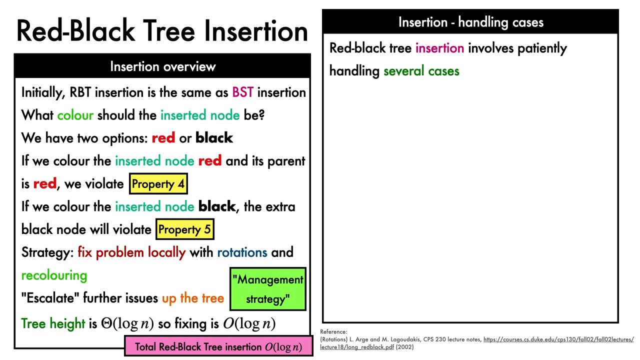 of log n. If we combine this fixing cost with the cost of insertion into a red-black tree, which we know is approximately balanced, we find that total red-black tree insertion is big O of log n. Let's now turn to the insertion itself. Red-black tree insertion involves patiently handling several cases. 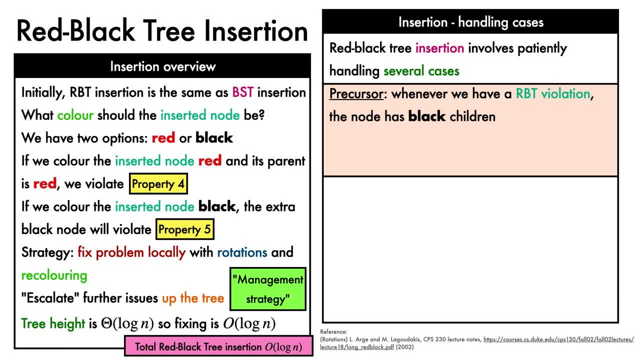 As a precursor before stepping through the cases, note that whenever we have a red-black tree property violation, the node in question has black children. We know that this is always true immediately after making an insertion, since nil nodes are black. It is also true when we look. 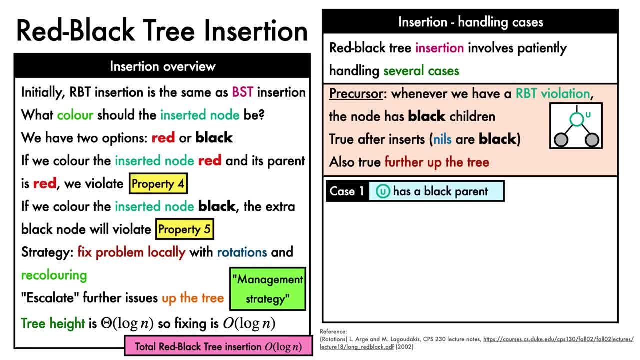 further up the tree. The first case we consider is when our issue node u has a black parent, a situation that looks like this From our precursor statement: u's children are black, so t1 and t2 are subtrees with black roots. 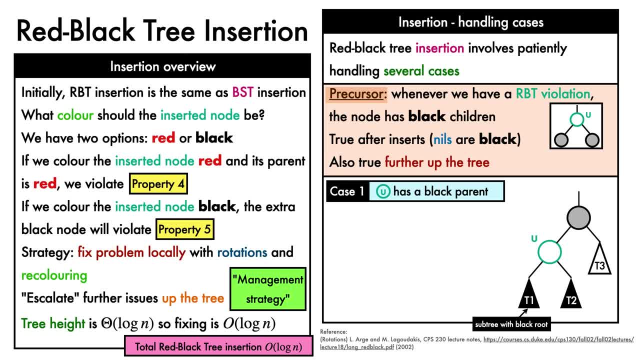 From now on, we'll use the notation of black-filled triangles to indicate subtrees with black roots and white triangles to indicate subtrees that can have red or black roots. The solution here is to simply colour node u red, Since u is not the root. we know that we have not. 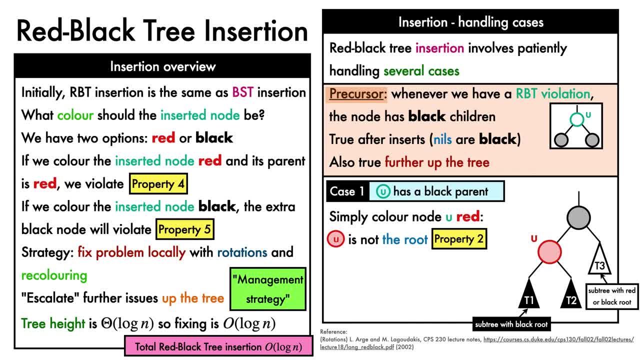 violated property. 2, the need for the root to be black, Since u only has black children. we have not violated property. 4, the need for red nodes to have black children, And since no extra black nodes have been added, we have not violated property. 5, the need for the same number of 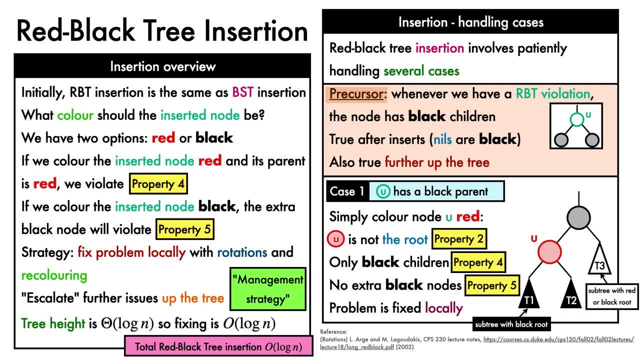 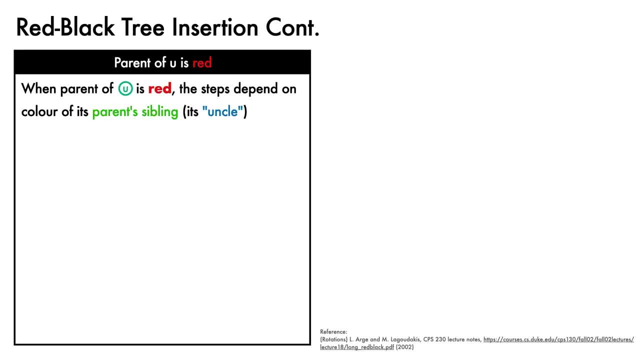 black nodes on each root-to-leaf path. Thus the problem is fixed locally, with no need for escalation up the tree. When the parent of node u is red, the steps to be performed to resolve red-black tree property violations depend on the colour of its parent's sibling. 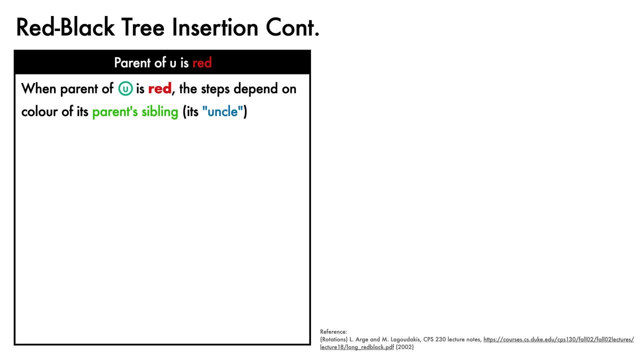 which by convention is referred to as its uncle. We'll first examine this problem as an example. first examine the case where u has a red parent and its uncle is red, which looks like this: Here the node with key p is the uncle of u. W indicates the grandparent of u. We handle this by pushing. 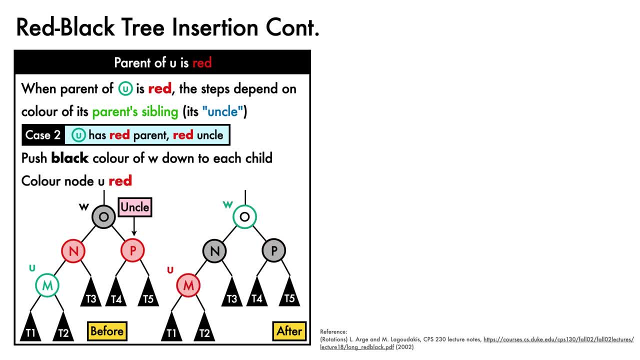 the black colouring of w down to each child and colouring node u red, We can see that we're fine on property 2 because u is not the root, on property 4 because u has black children and property 5 because the total number of black nodes in each path has not changed. Note that we 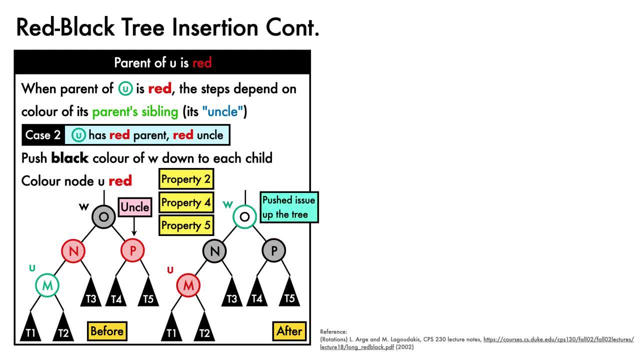 have effectively pushed the problem up the tree where it can be dealt with recursively. We now come to the third and most complex case to handle. u has a red parent and a black uncle. Part of the complexity is that this involves handling two sub-cases: The first, which we'll call case 3a. 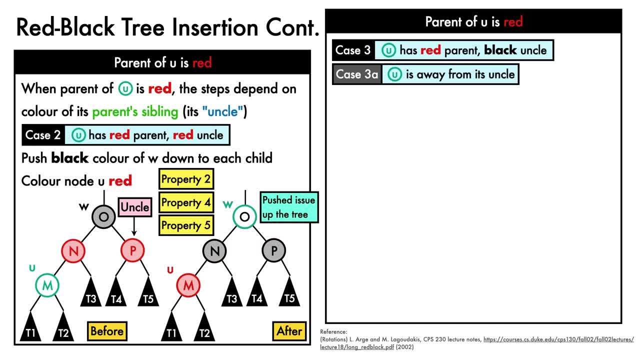 is the case when u is on a branch that is away from its uncle. It looks like this: where again, the node with key p is the uncle of u. Starting from this layout, we first apply a right rotation to w, then we colour. 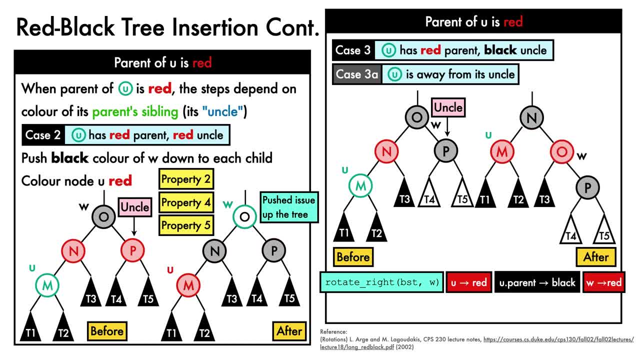 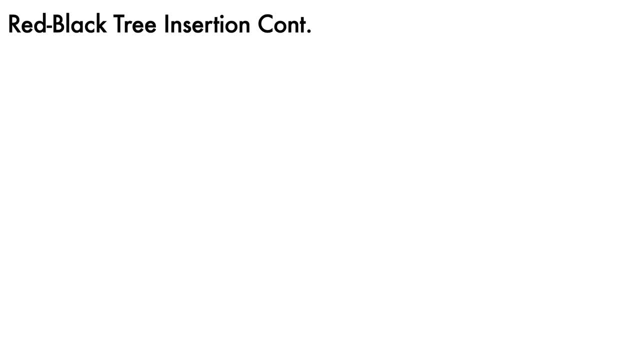 u red, we colour u's parent black and we colour w red. Note that, since we've only used a rotation to make changes, the binary search tree property still holds. We also see that all properties are satisfied, so the problem is fully fixed and no further escalation is required. We now come to 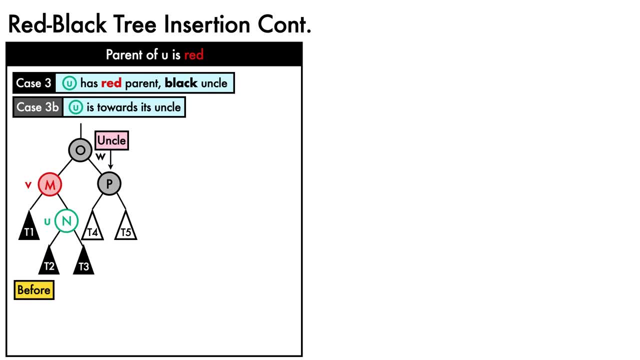 case 3b, where u is towards its uncle, which looks like this: Starting from this, our first step is to apply a left rotation to v, then a right rotation to w, to balance the structure. This time we recolour u black and recolour w red, As in case 3a. the problem: 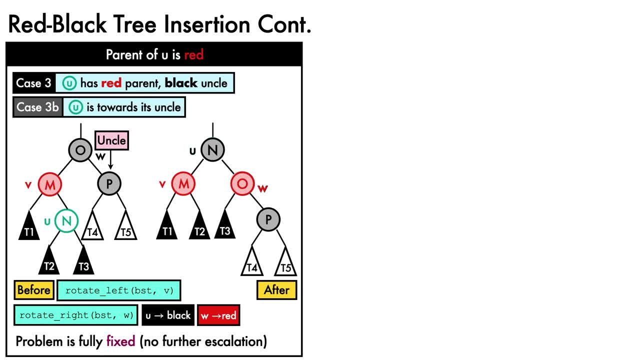 is now fully fixed and no further escalation is needed. Our fourth and final case is when u has no parent, like this. Here we simply colour node u black, which we can see will satisfy property 2 because the root itself is black and property 5 because the total number of black nodes in 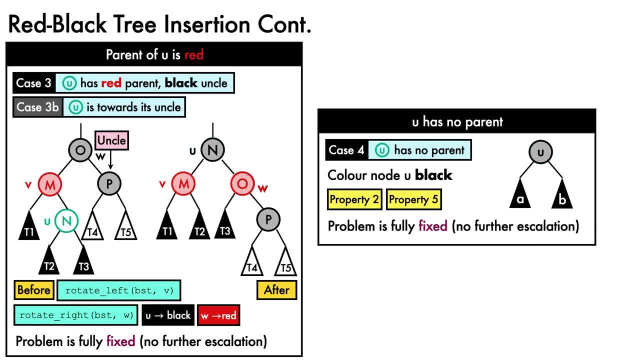 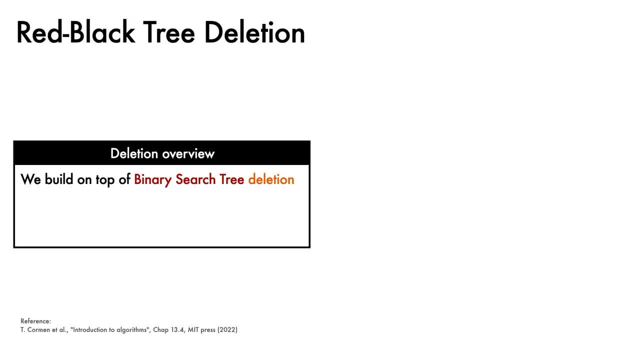 each path remains equal. As with case 3,, we have fully fixed all red-black tree property violations, so no further escalation is needed. We now turn to red-black tree deletion, which builds on top of standard binary search tree deletion. Unlike typical binary search tree deletion, however, 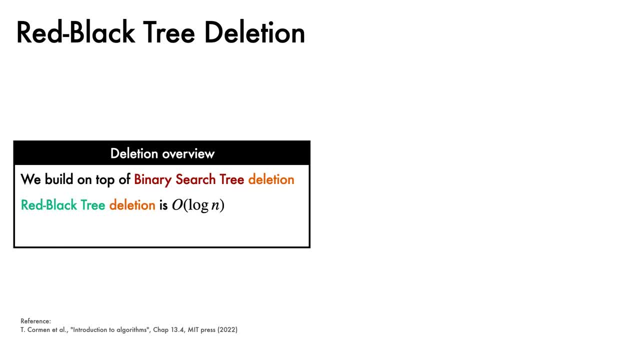 thanks to the balancing, we are guaranteed that red-black tree deletion is big O of log n. Before launching in, please prepare yourself mentally for the fact that it is quite complicated to do so. Just as with binary search tree deletion, the first component we'll define is a function. 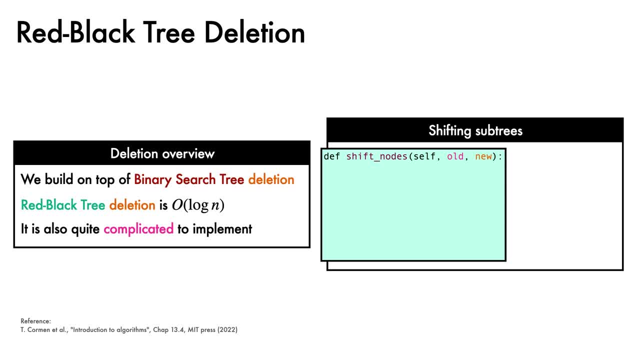 to shift a subtree from one location to another. For this we define a helper function which takes in three arguments: self, which is an instance of a red-black tree, the old node whose subtree will be replaced, and the new node that forms the root of the subtree that. 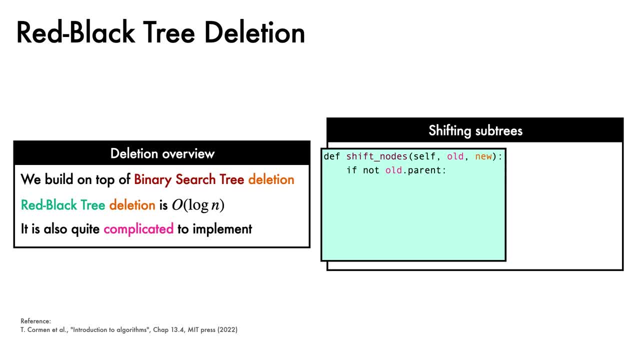 will replace it. If the old node has no parent, then it was the root. so we update the root to point at new. If the old node was a left child, we update its parent's left child to new. Otherwise it was a right child and we update its parent's right child to new. 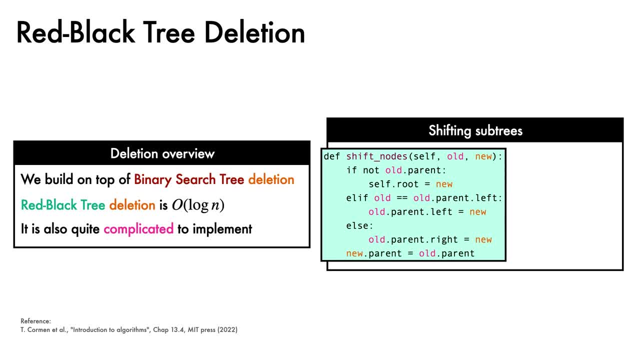 Finally, we update the new node's parent to the old node's parent. We'll show how this works on a simple tree where our function call requests that the subtree rooted at the old node with key 2 is replaced by subtree rooted at the new node with key 1.. For simplicity, we'll ignore red and 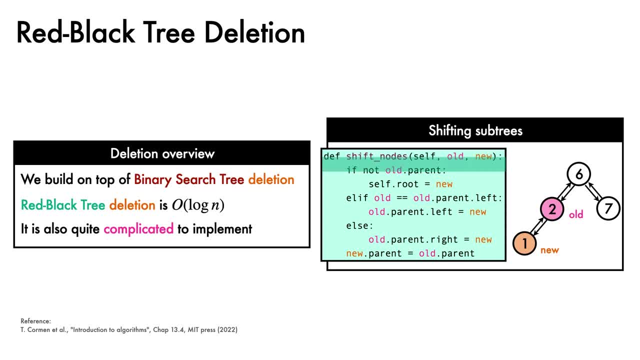 black colours here, since those will be dealt with elsewhere. We first check if the old node has a parent, indicating that it was not the root. It does have a parent. so we next check if it is a left child It is, so we move new up to replace it. Finally, 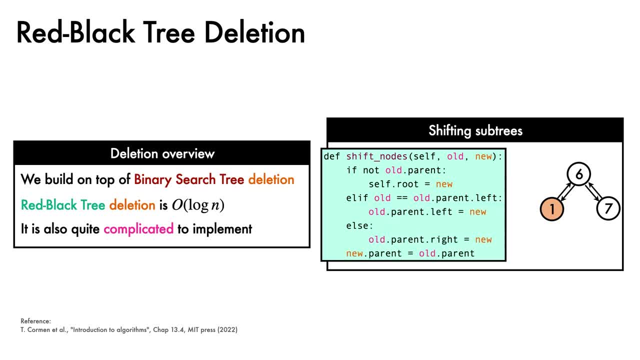 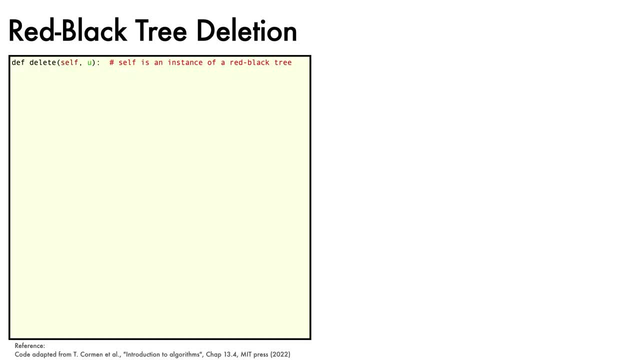 we update new's parent attribute to point to the old node's parent. To give some scaffolding to red-black tree deletion, we'll step through python code for the delete function which takes in a reference to self which is an instance of a red-black tree and you the node to be deleted. 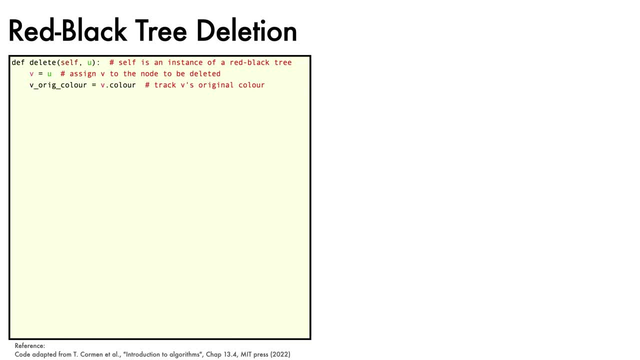 We first assign v to the node to be deleted and define a variable to keep track of v's original colour. What we do next depends on the children of u. If u's left child is nil, we apply some logic to shift its left nil child up. If u's right child is nil, we apply similar logic to shift its. 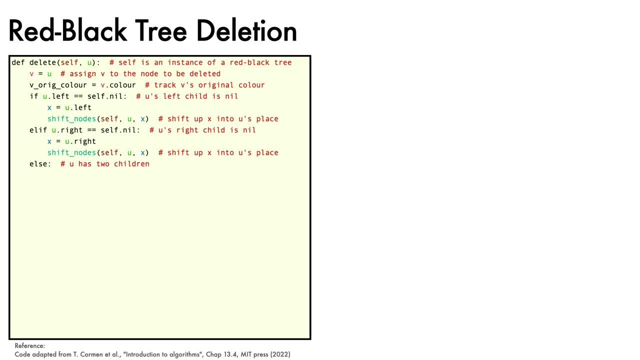 right nil child up. If u has two children, we apply some slightly more complicated processing that we'll step through shortly. Finally, whichever case we fall into, if v's original colour was black, we call a further helper function with x as an argument that fixes. 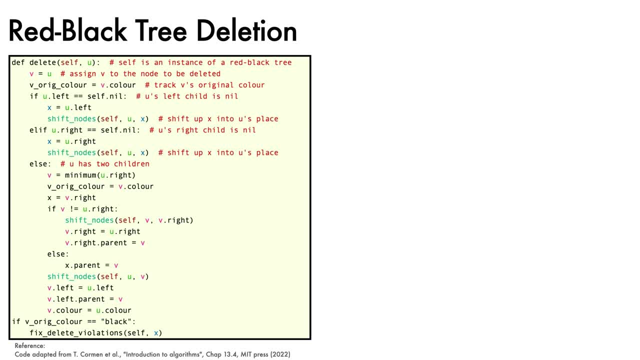 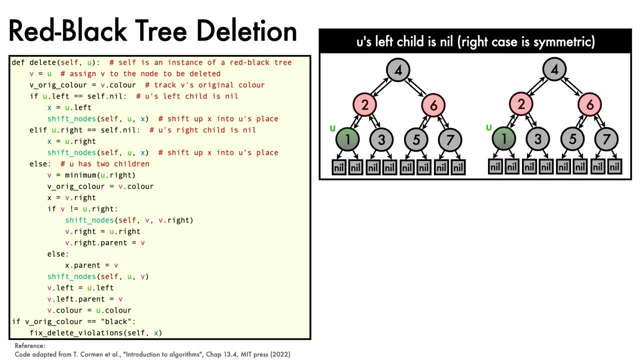 the violations to the red-black tree that have arisen. To illustrate this function at work, suppose that this is our red-black tree and u. the node to be deleted has q1.. Replicating this for clarity, we can see that the first steps of our function assign: 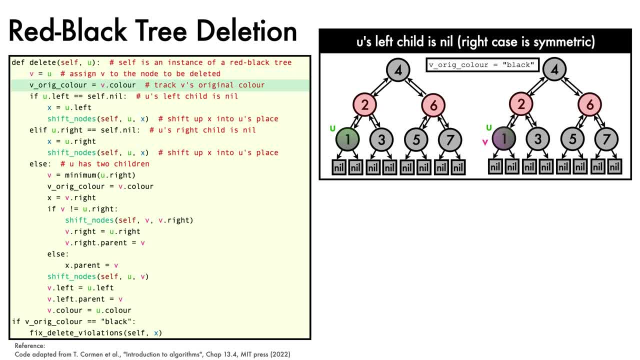 v to the same node as u and determine that v's original colour was black. Now we hit the conditional which evaluates to true, since u has nil as its left child. Then we assign x to u's left child, shown here, which is nil, and use our shiftNodes function to shift. 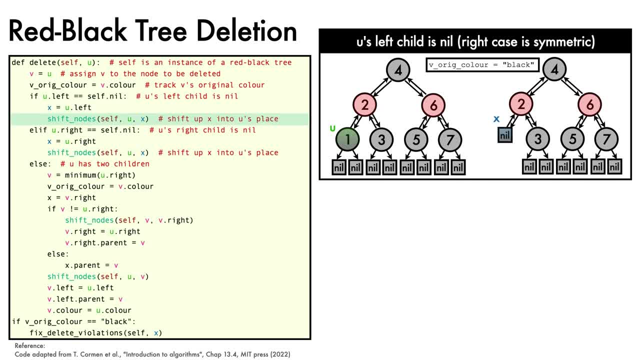 x into u's position, which gives us x to the left child and x to the right child. This causes u's right child to be dropped, Since v's original colour was black. we call fixDeleteViolations passing x as an argument. We'll explain how that works later. 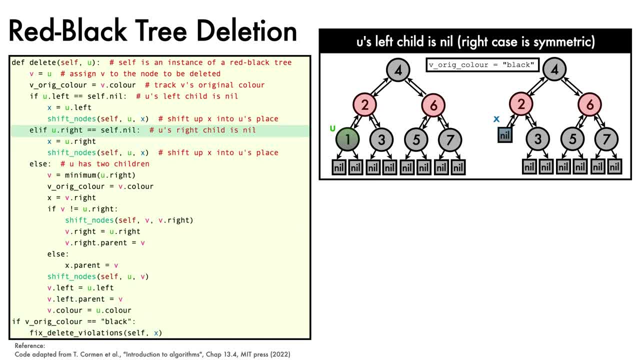 If, instead, we had found that u's right child was nil, we would apply symmetric logic, assigning x to u's right child and shifting x up into u's place. Let's now turn to the interesting case when u has two children. Here we'll pick the node with key 2 as the node for deletion. 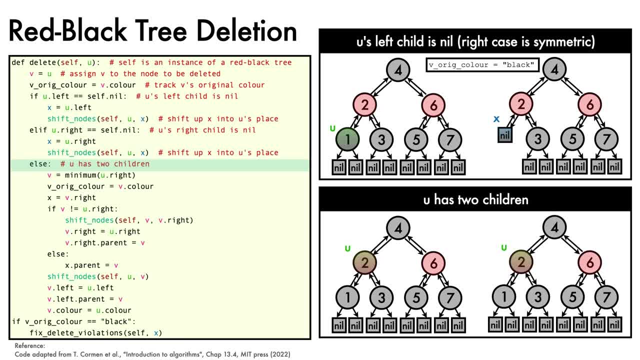 As before, we'll replicate. Our next step is to assign v to the successor of u, which we can do by calling minimum on its right child. in this case, giving that v is the node with key 3.. As above, the original. 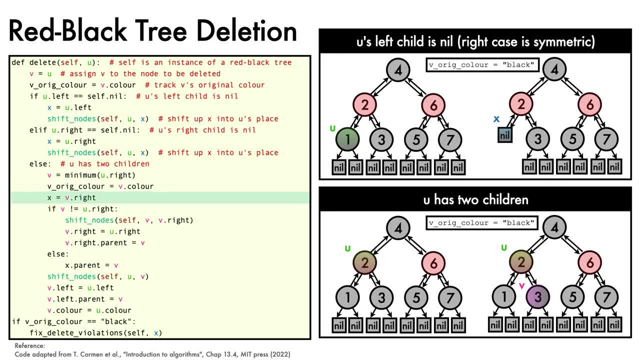 colour of v is black. Now we assign x to v's right child like this: If v was not u's right child, we'd need to do some more node shifting, like we do in typical binary search tree deletion. However, here it is u's right child, so we jump to the else statement and assign x as: 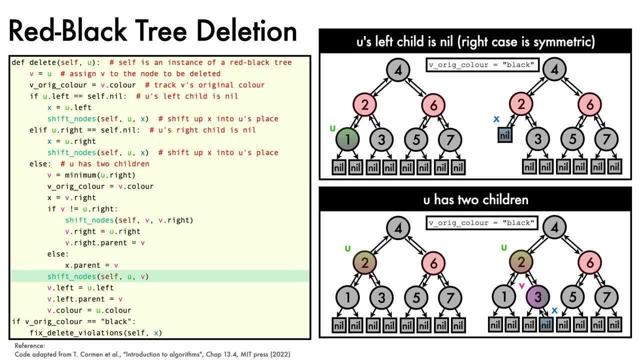 the node for deletion, which we do here Now we call shift nodes. to move v into u's place, We reattach u's left child as v's left child and point the parent attribute of this node back to v. Finally, we assign: 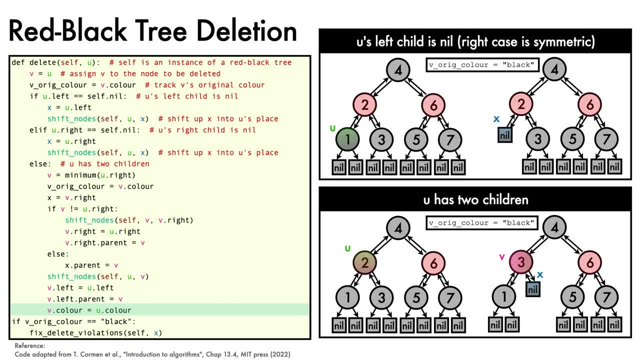 v's colour to match u's, which was red As before. since v's original colour was black, we call our helper function to help fix red black violations. You may reasonably ask: why do we only fix issues when the original colour was black? 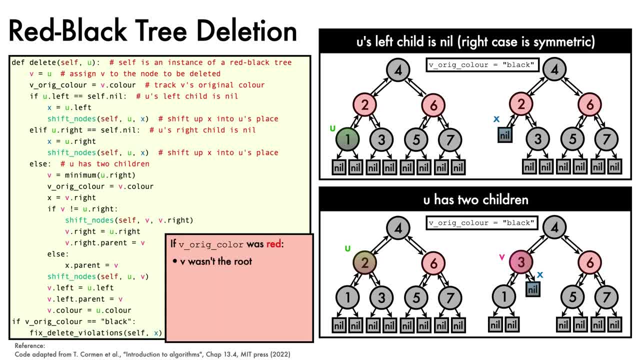 That's because v's original colour was red. v wasn't the root, so we haven't broken property. 2. No red nodes have become neighbours, only black nodes have become neighbours, if any. so we're fine on property. 4. Finally, the number of black nodes on paths from the root. 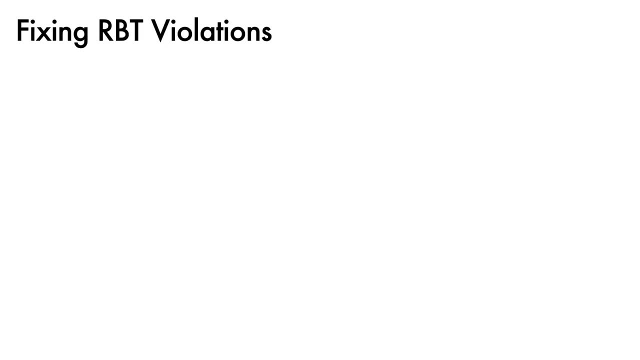 to leaves haven't changed, so we're fine on property 5.. We now turn to the process of fixing red black tree violations with our helper function. Since v was originally black, moving it will break property 5, as different paths will contain. 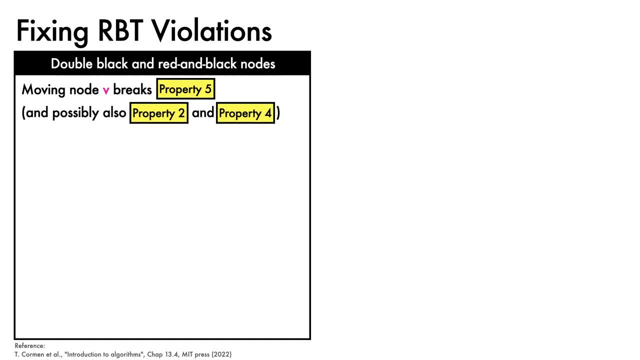 numbers of black nodes. It may also break property 2 if it caused a red child to become the root, and property 4 if it caused a red node and its parent to become adjacent. The slightly odd trick used here to resolve these violations is that when v is moved, 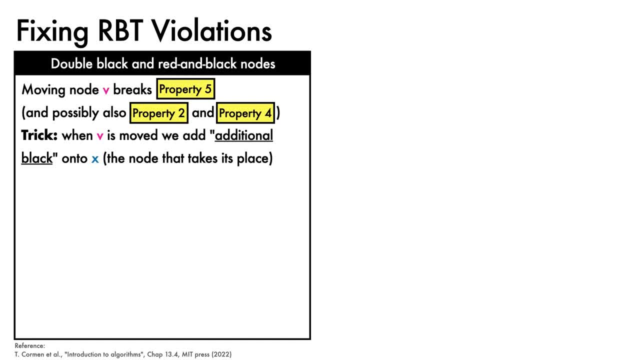 we add an additional black count onto x, the node that takes its place. This means that x is now either double black, if we added a black onto a black node, or red and black if we added a black onto a red node. This fixes the problem. 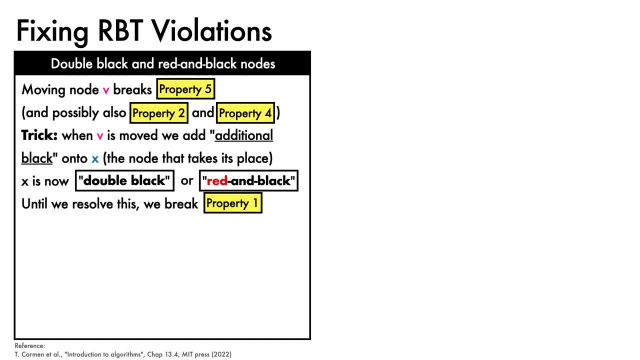 This fixes property 5.. However, until we've figured out how to resolve this new double node, we break property 1, which says that every node in the tree must be either red or black. To address this, our fixDeleteViolations function iteratively handles various cases. 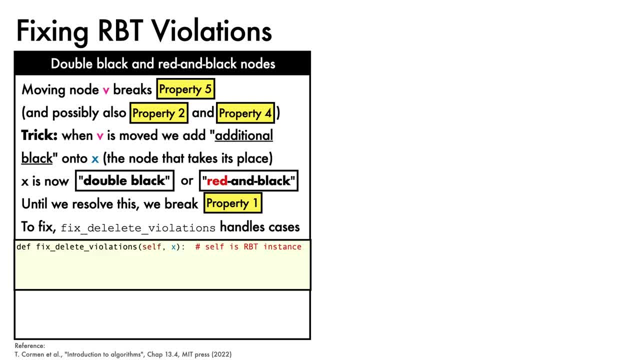 that can arise until all violations are resolved. The fixDeleteViolations function takes self as an argument, which is an instance of a red black tree and x the problematic node. Then, while x is not yet the root and its colour is black, we can now fix the problem. 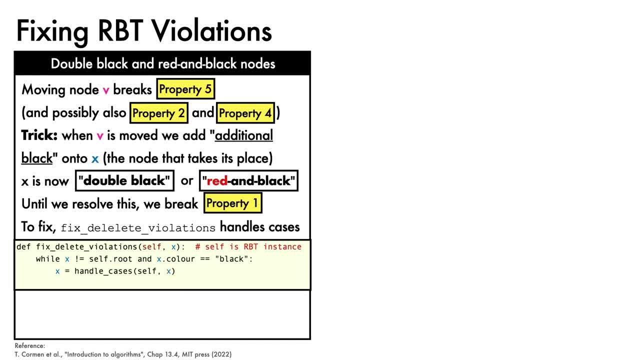 We apply transformations for various cases and update x accordingly. where inside the while loop x is a double black node? Finally, when the while loop exits, we set x's colour to single black. The cases we handle depend on the colour of x's sibling. 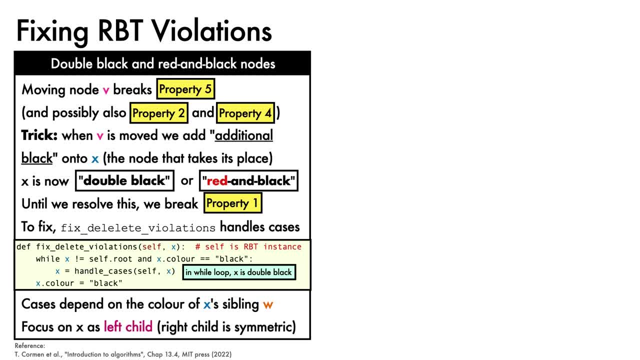 which we'll refer to as w. We focus on the four cases when x is a left child. The cases when it's a right child are symmetric, with each of the four cases addressed symmetrically. Case 1 considers the setting when x's sibling doubles with x's sibling. We apply transformations. 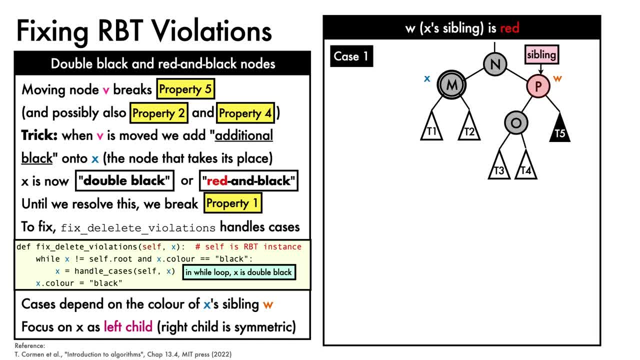 for various cases and update x accordingly. where inside the while loop x is a double black node and x's sibling w is red, Here we've used a second circle to indicate that x is double black. As before. the triangles denote subtrees where white subtrees can have. 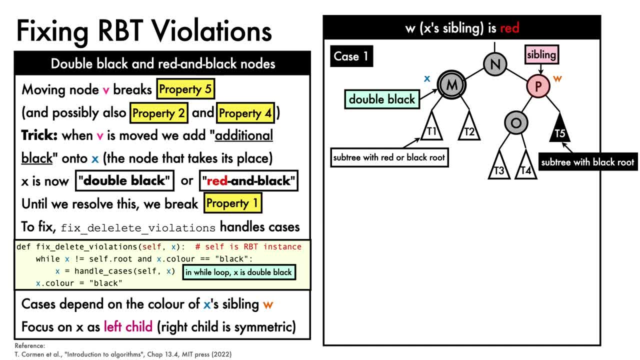 either a red or black root, while black subtrees have a black root. Starting from this structure, we add another variable, y, to point to the highest node locally, then call rotateLeftOnY to shift nodes over to the left. We then recolour y red and recolour w black, Since x has moved. 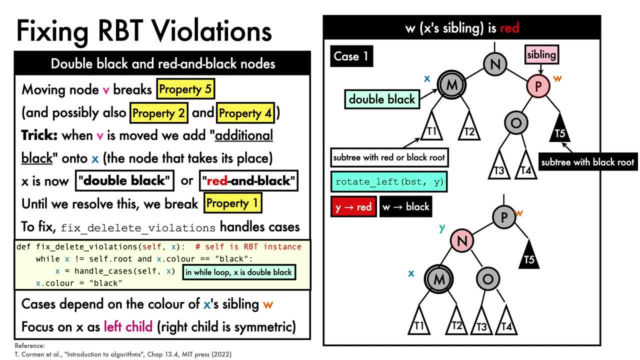 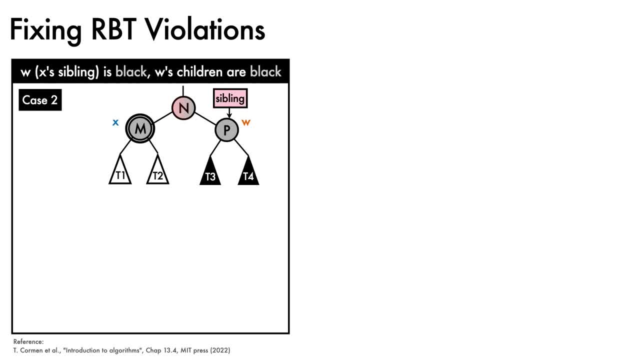 the node with key o now becomes its sibling, so we update w to reflect this. We now turn to case 2, where x's sibling w is black and both its children are black. In addition to using an extra circle to denote that x is a double black, we also use shading. 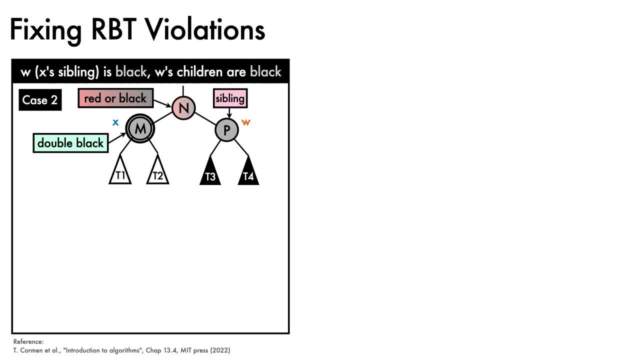 to denote that in this layout the top node can be either red or black. Starting from this, we first recolour w red and move x up by one with the corresponding extra black count. Now that x has moved up, we also drop the. 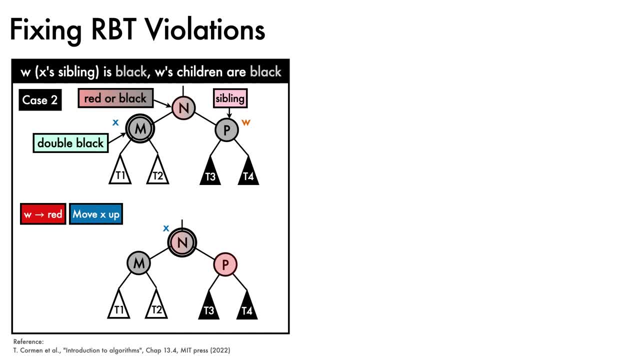 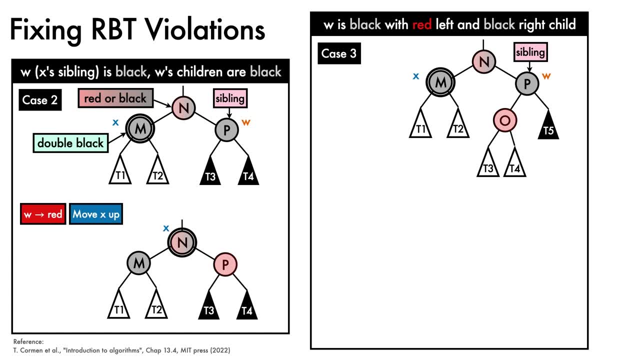 w variable since x's sibling is no longer among the visible nodes. In case 3, we consider when x's sibling w is black, with a red left child and a black right child. Starting from this layout, we first apply a right rotation to w to shift. 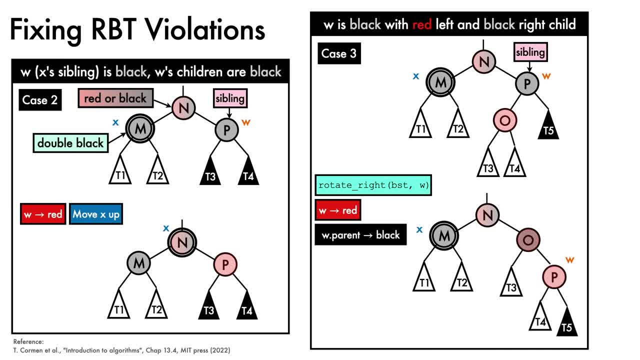 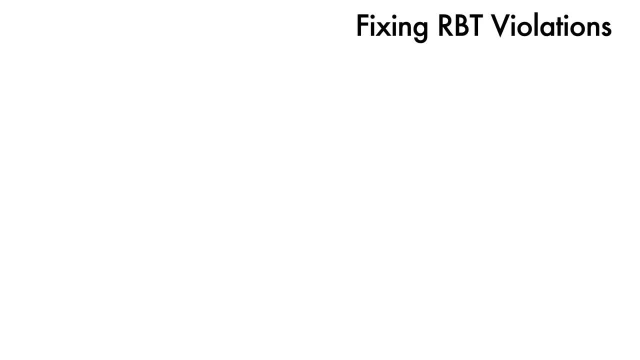 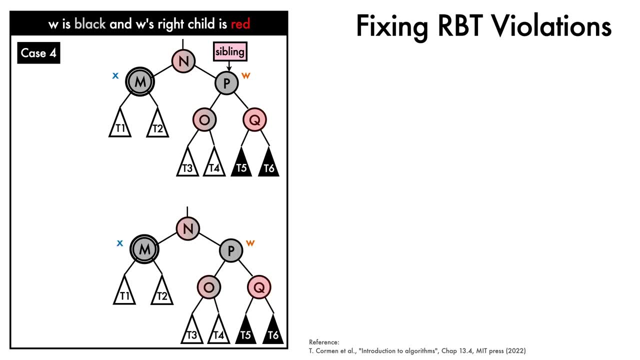 the nodes further right. Then we recolour w red and w's parent black. Finally, we update w to reflect the new position of x's sibling. We now come to the fourth and final case where x's right child is red. Starting from this, we first apply a left rotation on w to shift. 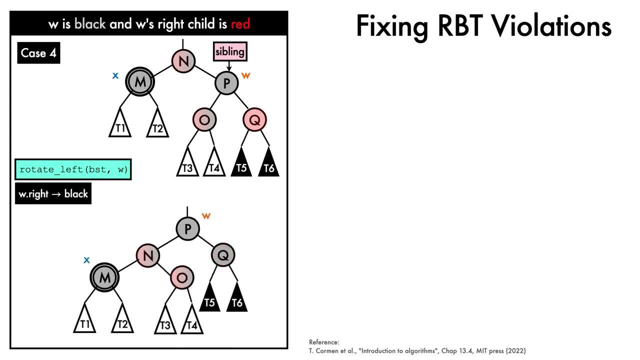 nodes over. Then w's right child is recoloured black, w is recoloured with its left child and w's left child is recoloured black, With the number of black nodes on the left increased by one. we can now thankfully get rid of the double black at x to restore balance. 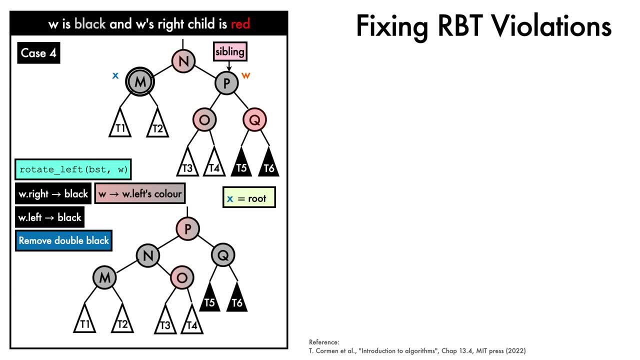 We set x to be the root and have no further use for w. Ok, we've looked at four cases, so let's summarise how they flow together. Let's start with case 3, where x's right child is red and w's left child is black.